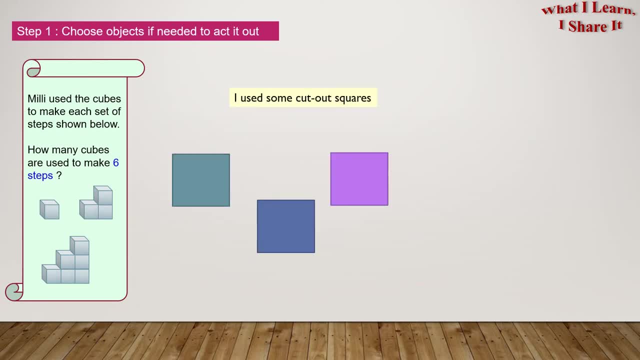 I used some cut-out squares. Step 2. Show what you know. So here is the one square for one step, And then here are the three squares for two steps, And here are the six squares for three steps. Step 3. Act out the problem. 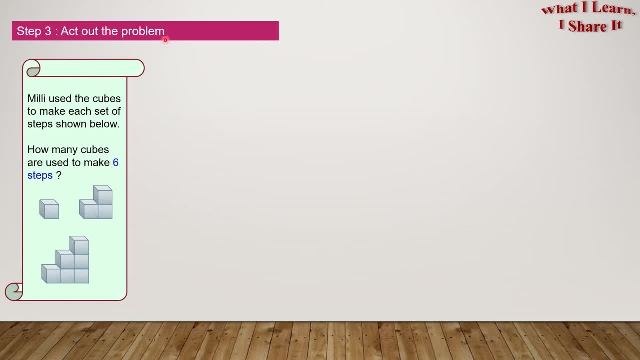 Since here we are, asked how many cubes are used to make six steps, we have to continue from the three steps and move on to four steps. So 10 squares for four steps, 15 squares for five steps And 21 squares for six steps. 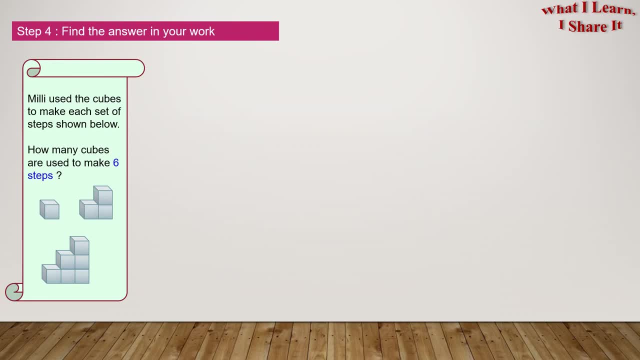 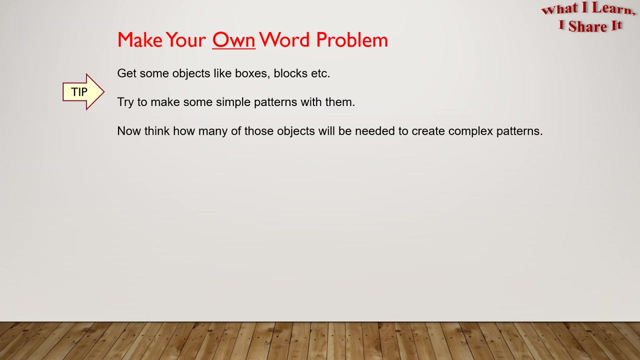 Step 4.. Find the answer in your work. So there are 21 squares for six steps. 21 cubes are used to make six steps. Yay, We solved the problem. Coming up is the fun part, and that is Make your own word problem. 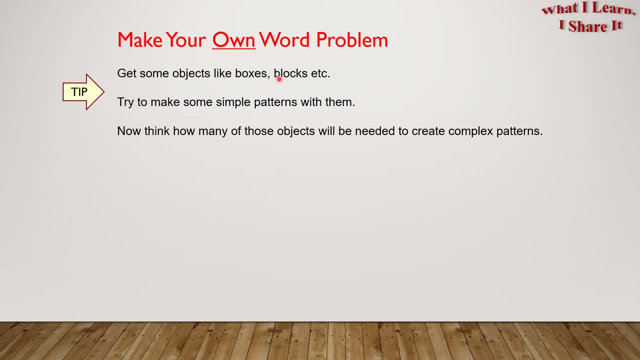 Here's a tip: Get some objects like boxes, blocks, etc. Now try to make some simple patterns with them. Now think how many of those objects will be needed to create complex patterns. Here's an example: Sam got some cans and made the patterns like this: 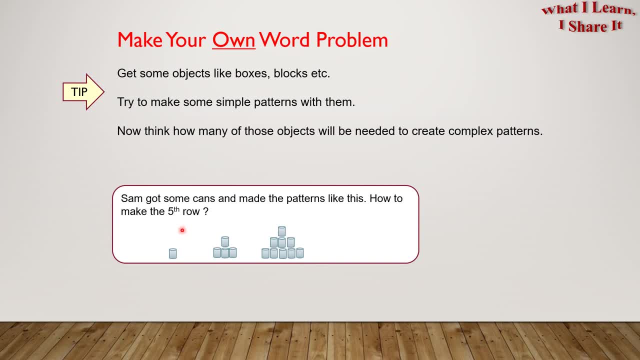 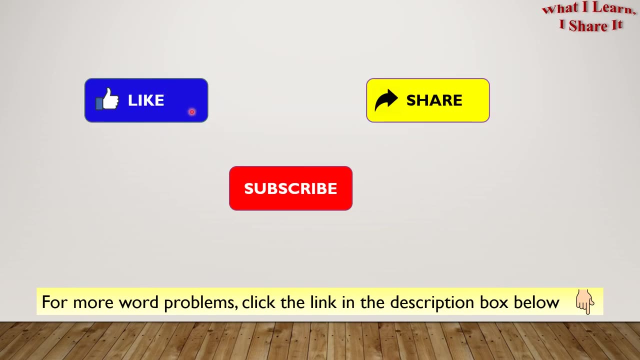 How to make the fifth row So exciting to make our own word problems. For more word problems, click the link in the description box below. Hope you like my video. Thanks for watching. Please like, share and subscribe to my channel. See you, Bye.